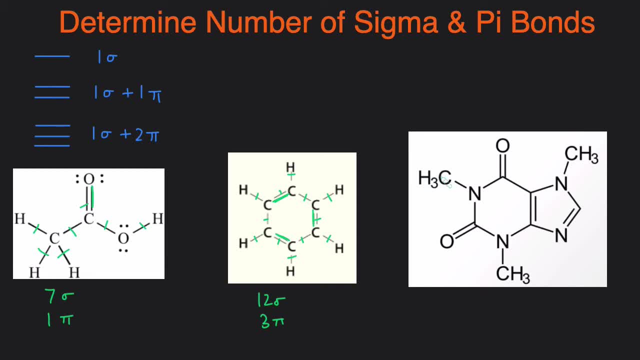 This one's a little bit different, Because then it shows you it's a CH3, but it doesn't show you the individual bonds. So what we're going to first do is just draw out the three H's: One H bond, another H and then a third H. 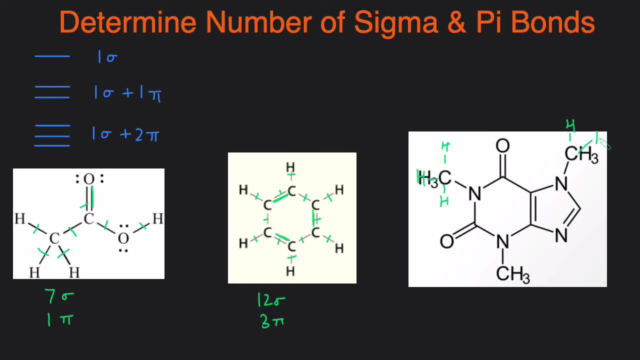 And then this one's also CH3, so we'll have one H attached, another H attached and a third H attached. When you draw it out this way you can see the specific number of bonds and it will be easier to count the number of sigma pi's. 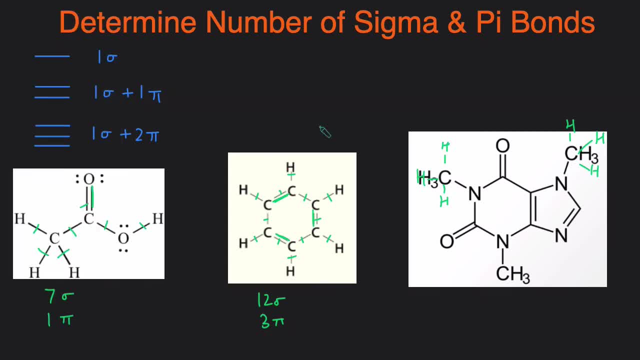 Then we're going to count the. Let's switch up the colors. So now we're going to count the number of sigma bonds. And remember there's a sigma bond in every type of bond, So 1,, 2,, 3,, 4,, 5,, 6,, 7,, 8,, 9,, 10,, 11,, 12,, 13,, 14,, 15,, 16,, 17,, 18,, 19,, 20,, 21.. 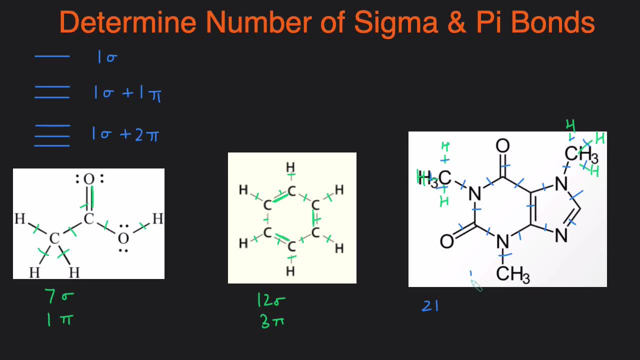 I have 21 so far, but I realize I've got to draw the CH3s here. So we're going to draw the three hydrogens attached to the carbon, And that'll be 22,, 23, and 24.. 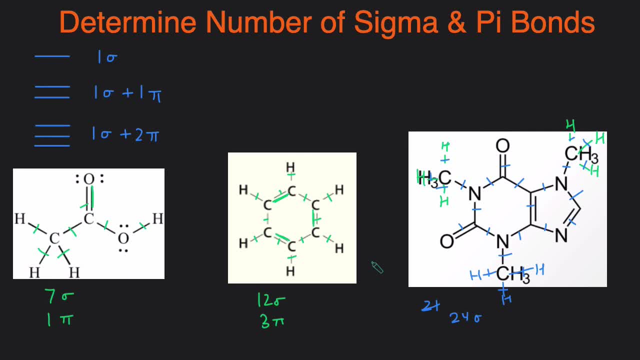 So that'll be a total of 24 sigmas, And then how many pi bonds will there be? There'll be 1,, 2, 3, 4 pi bonds, And that's it. That's how you can determine the number of sigma bonds and the number of pi bonds. 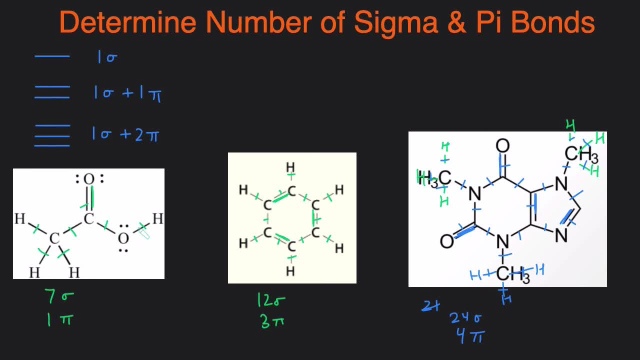 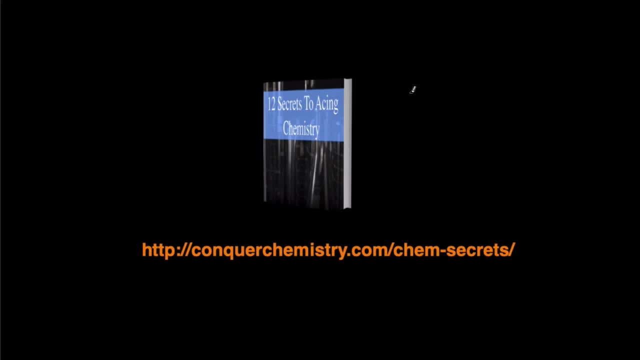 Just tick off one sigma for every type of bond, and then any remaining bonds will be pi bonds. If you want to learn how to ace chemistry, if you want to learn what's the best way to study for this class, if you want to learn some neat tricks and tips to take into your exam and do better on them, 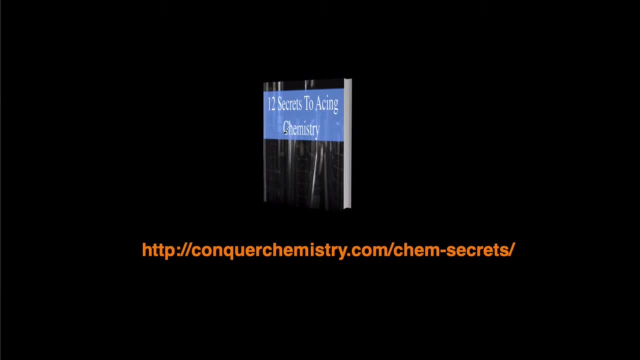 then you should head over to my website and get this free guide: 12 Secrets to Ace in Chemistry. You can head over to wwwconquerchemistrycom slash chemsecrets. I'm going to include a link in the description below. Check it out. 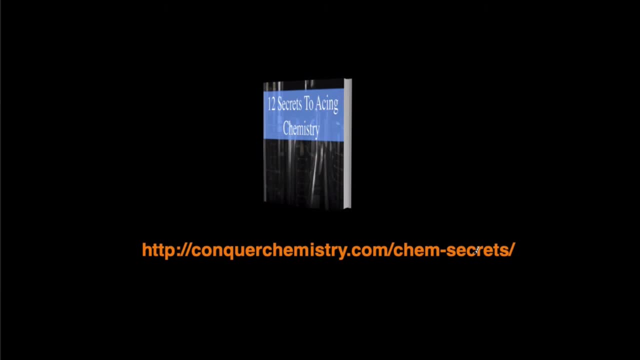 I think it's really going to help you and you're going to like it. Until next time, keep working hard and continue the good work.